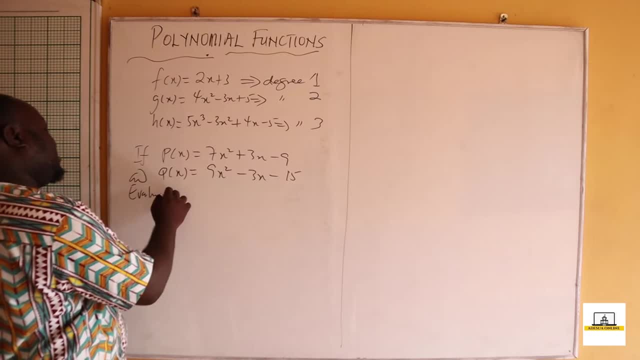 I add a polynomial of degree 3.. So this is a polynomial of degree 3.. So if I tell you, if p of x is equal to 7x plus 3x, squared minus 3x plus 5, this is a polynomial of degree. 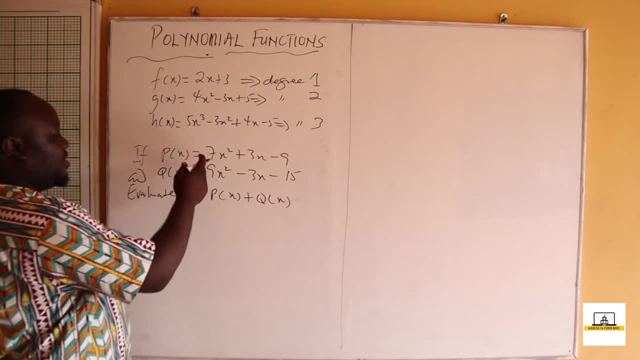 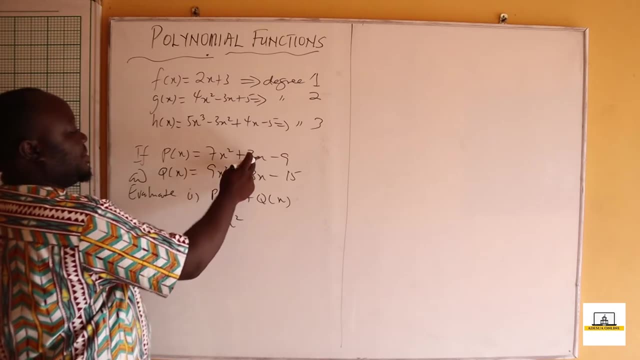 3. So if I tell you, if p of x equals to 7x plus 9 and q of x equals to 9x plus 10 and q of x equals to 9x plus 10. That is a polynomial of degree 3. This looks quite similar to last. 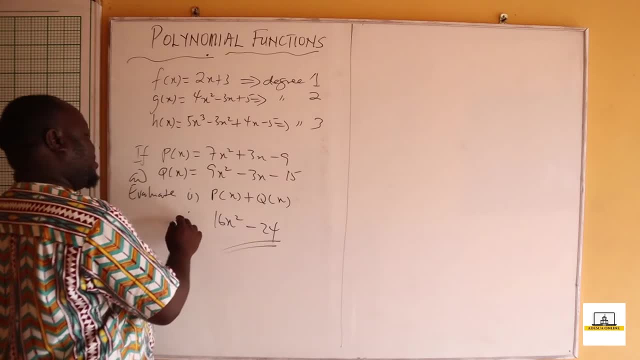 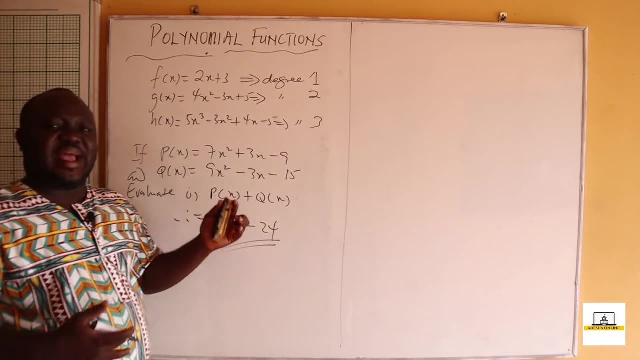 damage. So in thatórs. So yes, We have g. You can say this is equal to 16x squared minus 24.. Now, when we say addition and subtraction, we all know how to add and subtract, so I don't need to stress so much about this. 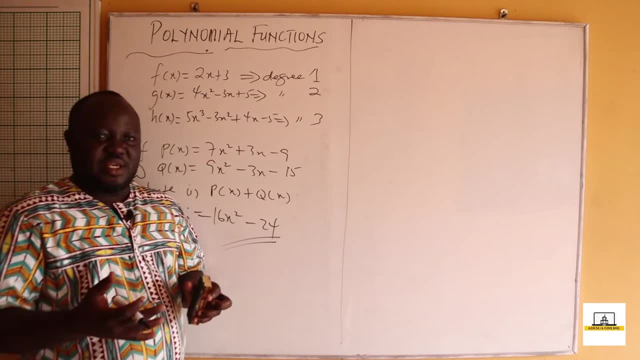 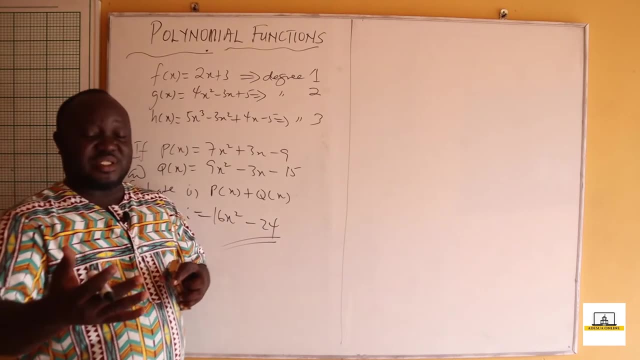 You understand. So you just add your like terms. If x cubed, we'll add x cubed, x squared, we'll also add x squared, x will add x and then constant will add a constant. But don't go and add 7x squared plus minus 3x. 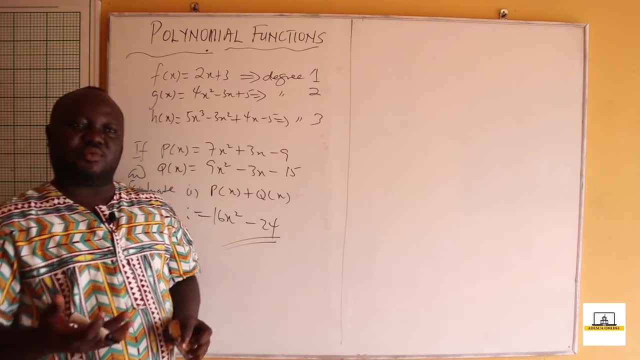 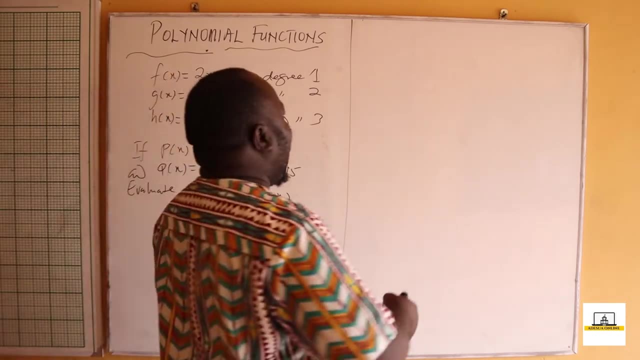 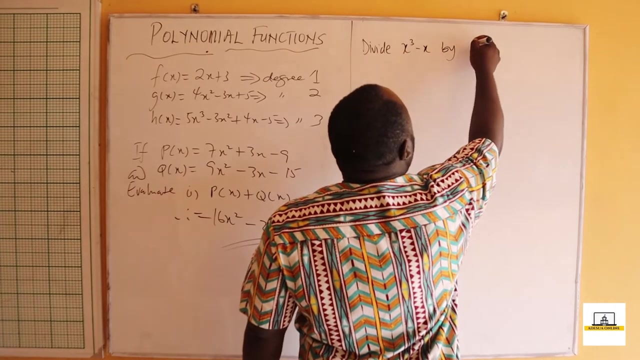 No, we don't do that, So each coefficient will add its corresponding coefficients. The same thing applies to subtraction. Now, when it comes to division, I'm going to ask you to divide x, cubed minus x, by, let's say, x plus 1.. 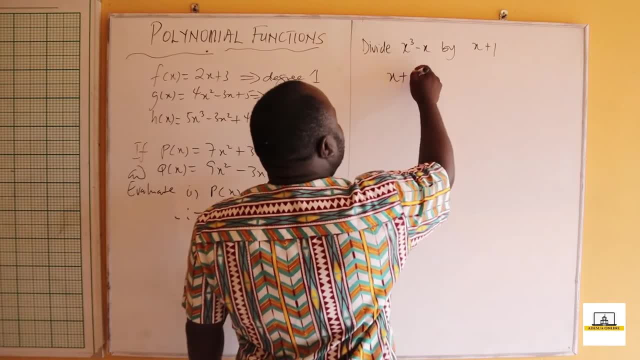 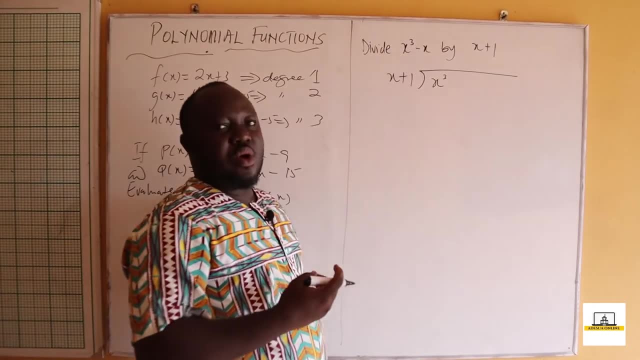 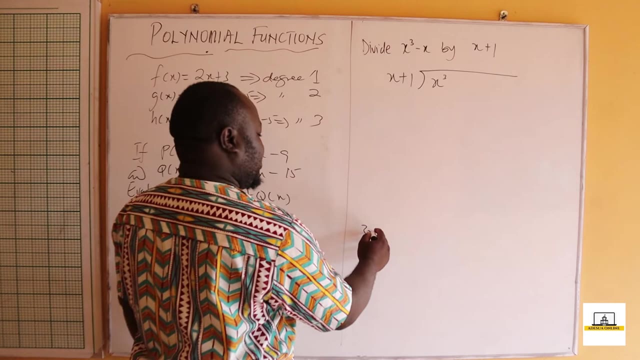 Now dividing this, we shall have x plus 1 divided by x cubed minus x. Now, x cubed minus x doesn't mean that there's no subtraction, It means the value of x squared, and so on and so forth. You know, if I have x cubed 3x cubed minus even 3,. 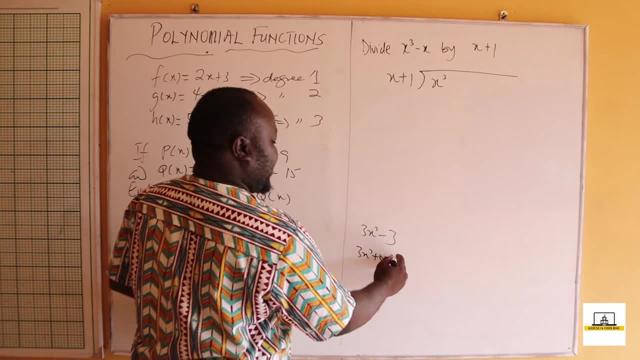 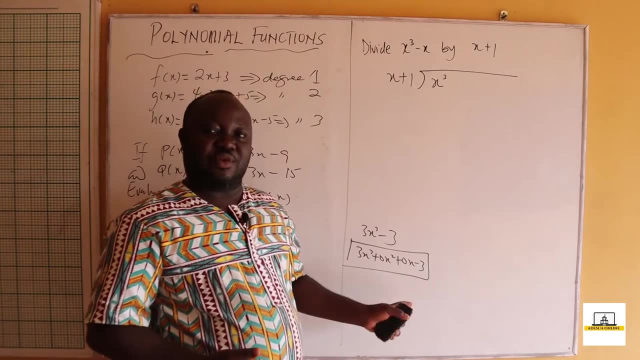 this means that this is 3x cubed plus 0x squared, plus 0x minus 3,. okay, The coefficients of x and x are also there, but just that they are zeros, okay. So x cubed minus x can be written as x cubed. 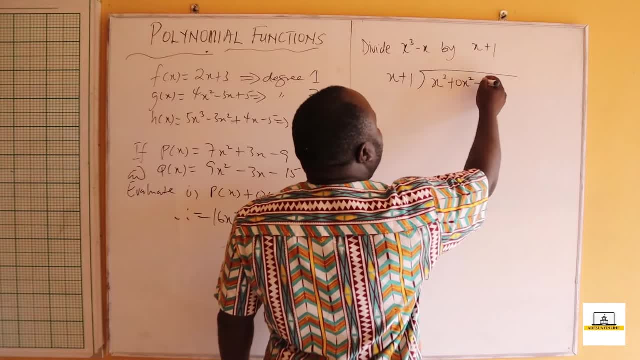 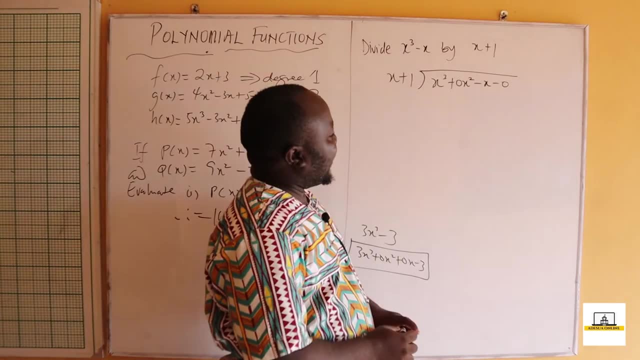 plus 0x squared, okay. minus x, minus what Zero Okay. So this means that we have x cubed minus x, where this is 0 and this is 0.. The constant is also 0.. So now we divide. 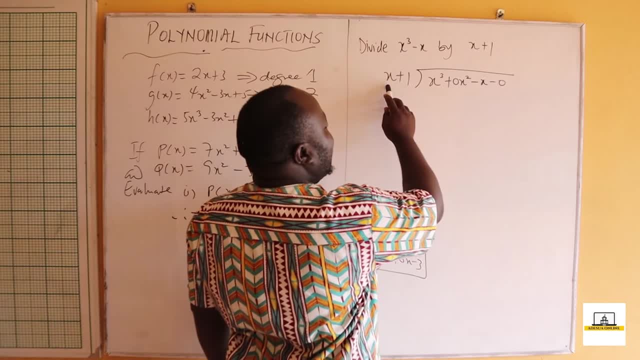 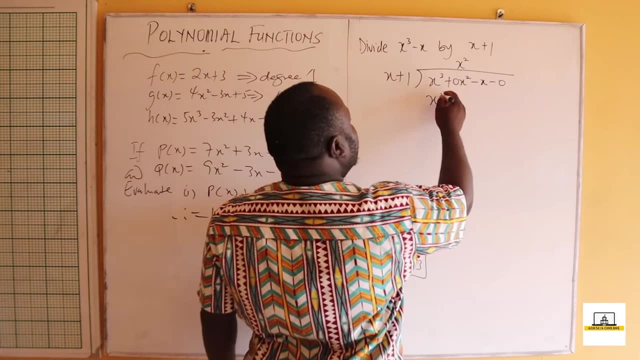 Now, if this is x and this is x cubed, what do I multiply with x to get x cubed? You told me, it is x squared, so I put x squared here. So x squared times, x is what X cubed. 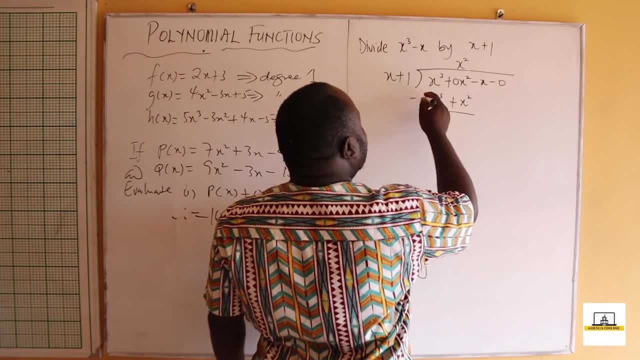 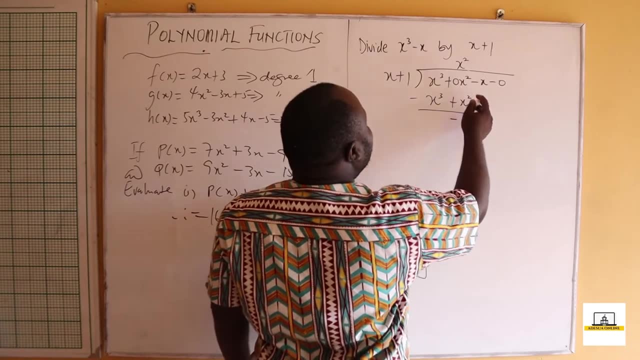 x squared times 1 is what x squared. okay, You subtract This will give me 0.. Now, 0x squared minus x squared will give me minus x squared. It's like having 0 minus 1.. You get minus 1x squared. 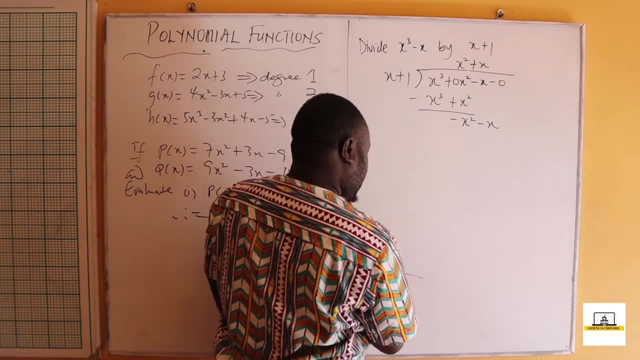 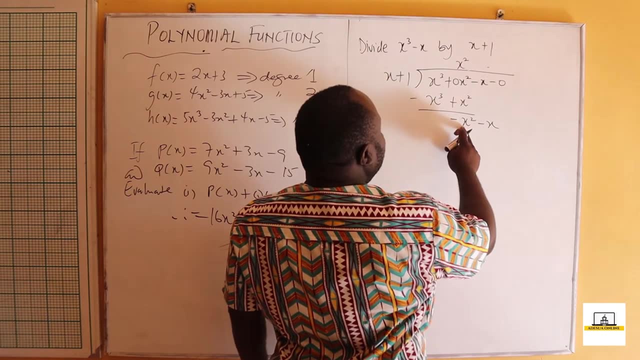 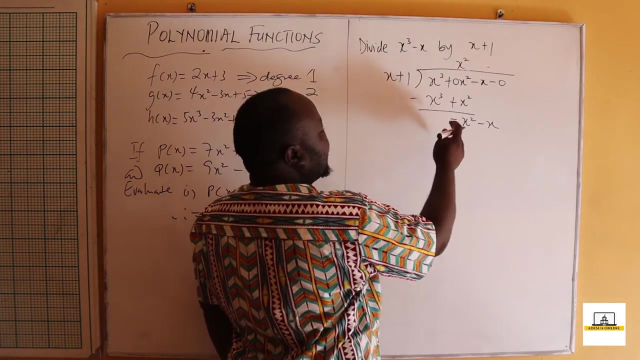 Then I bring my minus x down. So over here we shall have x squared times x is x squared, x squared times x is x cubed and x squared times 1 is x squared. Very good, So x cubed minus x cubed is 0,. 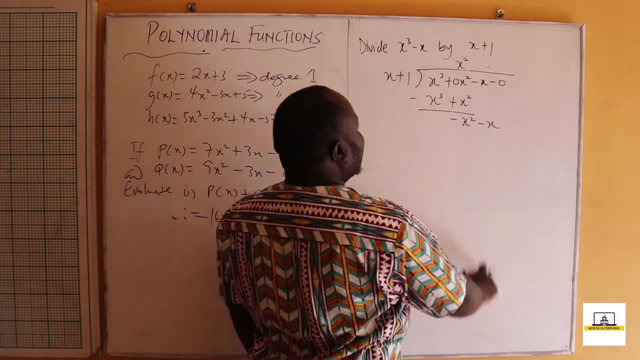 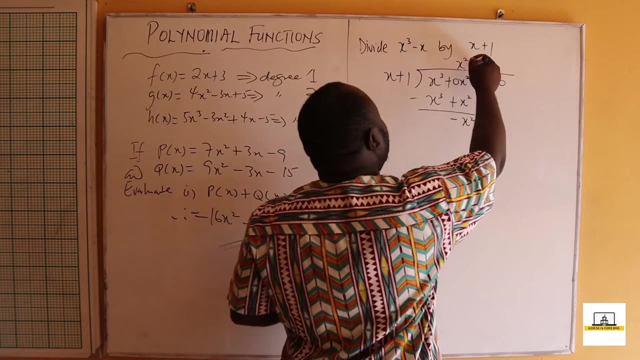 and 0x squared. minus x squared is minus x squared. Then we bring our minus x down. Now, if I have minus x and this is x, what do I multiply with minus x to get x? That will be minus x, okay. 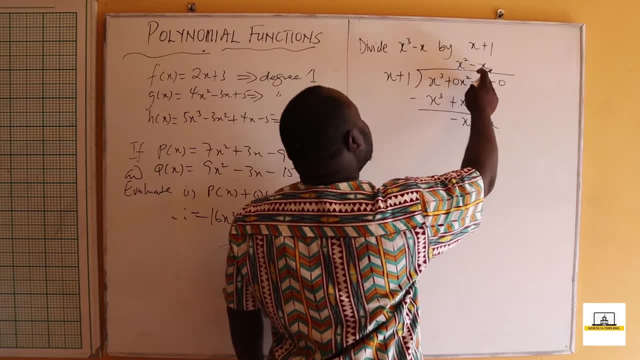 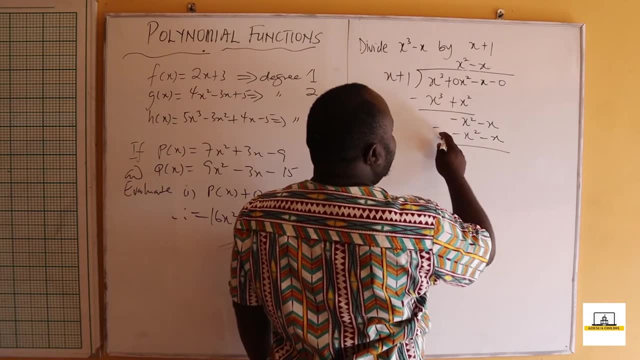 So what do I multiply with x to get minus x squared? It will be minus x. So minus x times x is minus x squared. Minus x times 1 is minus x. We subtract: This will give me 0, and this will also give me 0.. 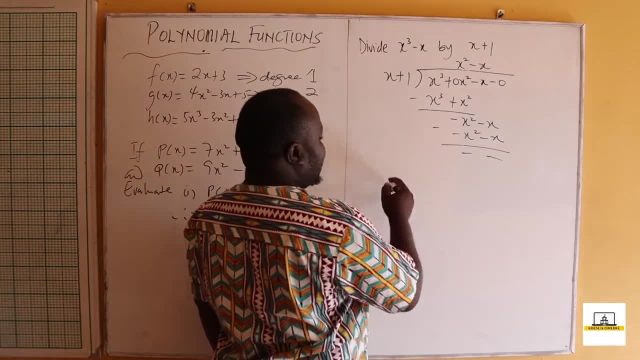 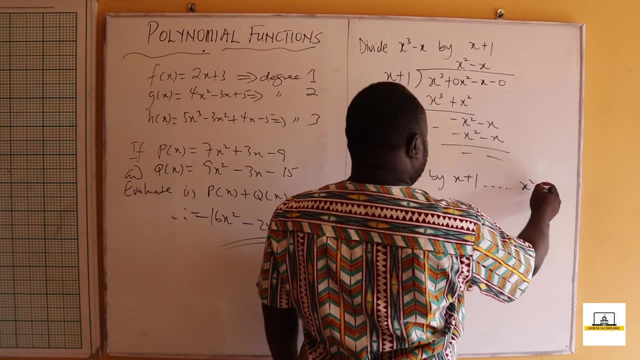 So I have 0, and this also 0.. So if I should divide x cubed minus x by x plus 1, I get a factor of what x squared minus 1.. My quotient is x squared minus x. okay. 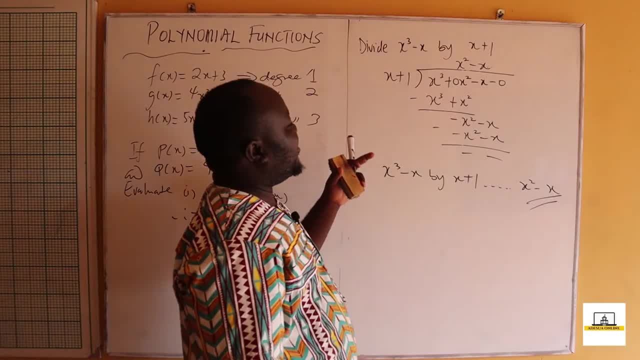 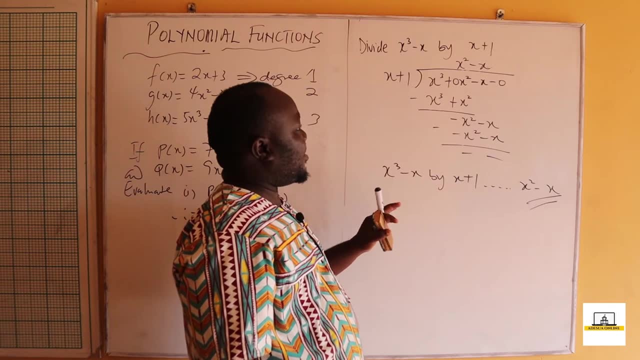 And it leaves a remainder of what 0.. So if we should divide x cubed minus x by x plus 1, it leaves a remainder of 0, and the quotient of what x squared minus x. So one thing you notice is: 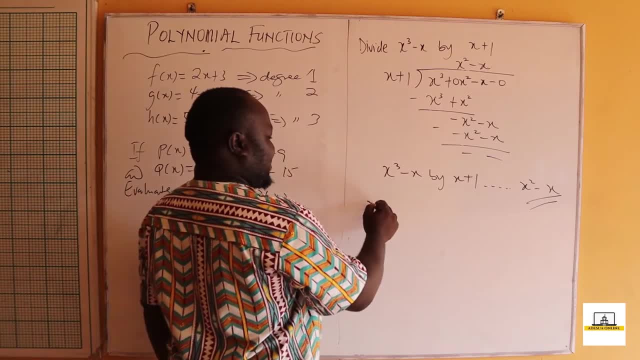 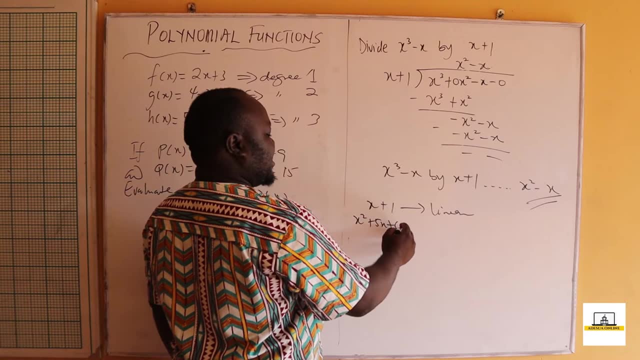 if you have a linear function, you have x plus 1, this is linear, okay. When you have a quadratic function, let's say x squared plus 5x plus 6, if you factorize it you get x plus 2, x plus 3.. 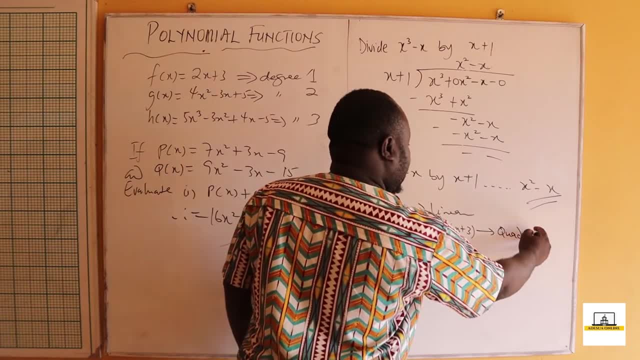 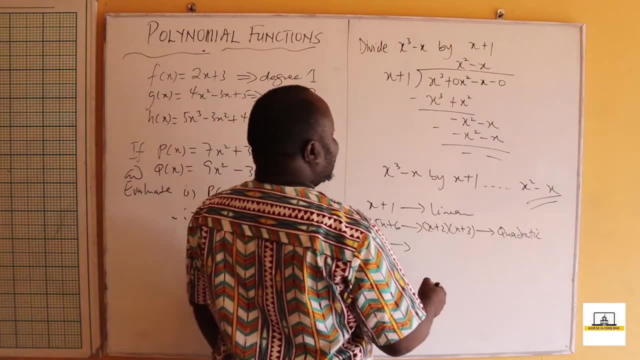 So this is also what Quadratic right. So if we have a cubic function- x, cubed minus x- okay, And once you factorize this, this will also give us x plus 1.. Then we shall also have, when you factorize x, as you have, x minus 1,. 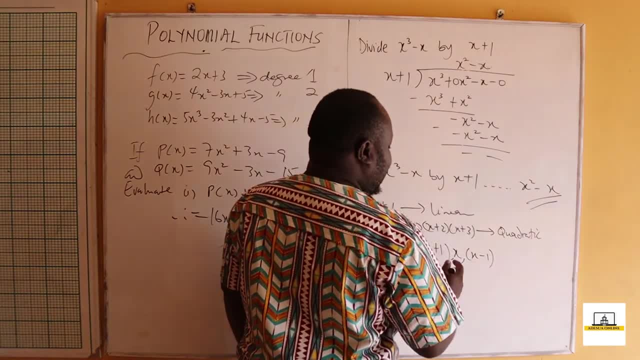 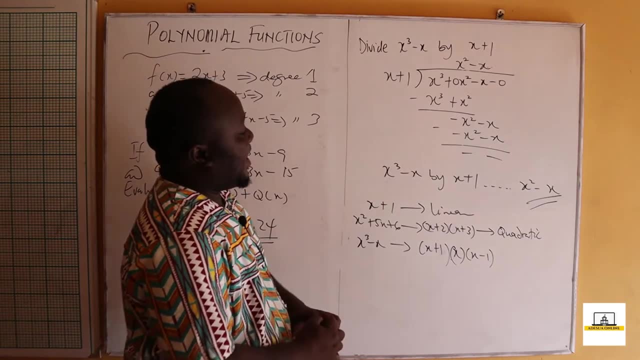 so x comma, then you have x minus 1.. So these are the three factors. If we should multiply, so we multiply this times, this times this. you get this okay. So we have what x cubed minus x? So this is a cubic function. 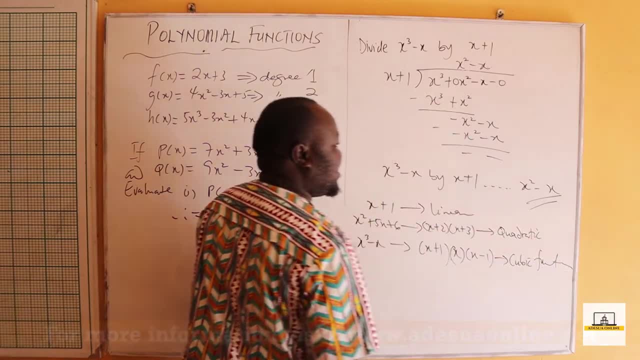 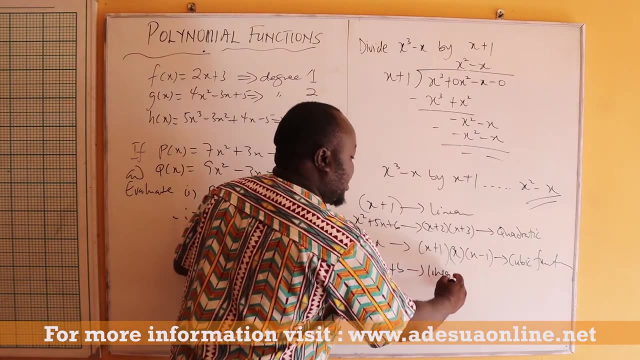 A cubic function. So what I'm trying to say here is: if you have a linear function, it means these factors are what a, x plus b for linear, okay, For quadratic we can have a x plus b. 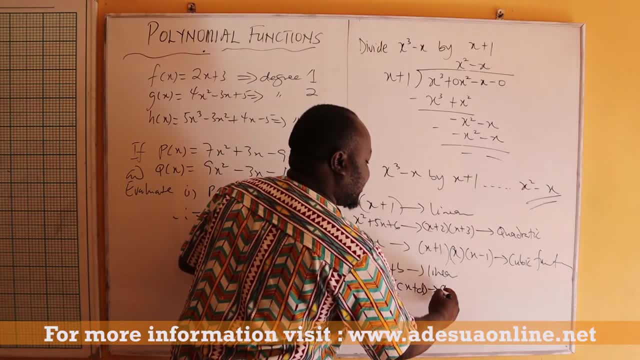 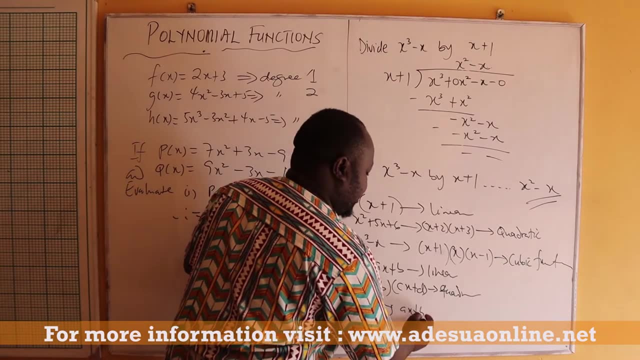 and then what: c x plus d. That is for quadratic And then for cubic there will be three factors. okay, So we shall have a x plus b, let's say c x plus d, and then e x plus what. 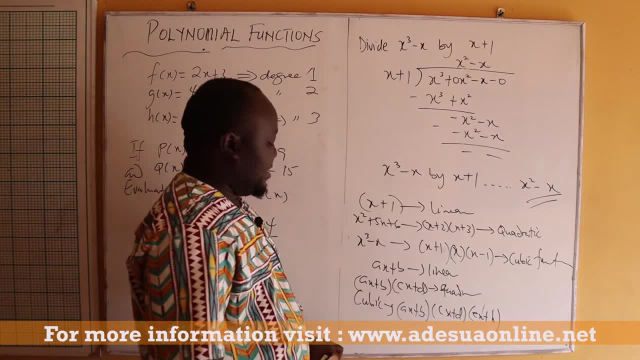 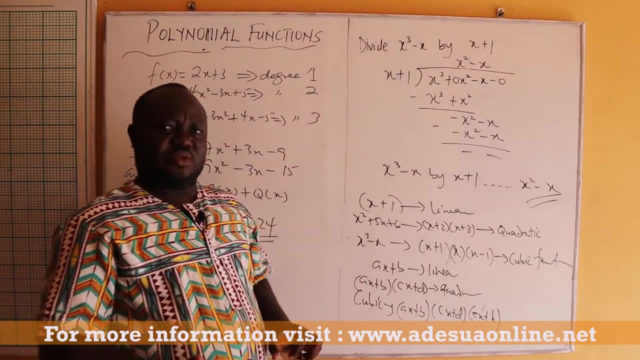 h. There are three factors when it comes to the cubic one. So for quadratic we have two, Linear we have only one. okay, So when we talk about a cubic function, okay, it means when we should divide it, we can get three factors. 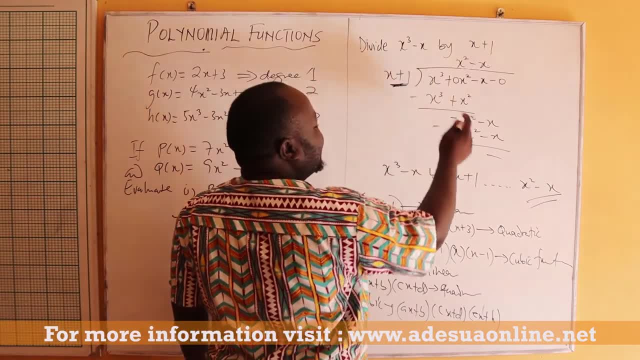 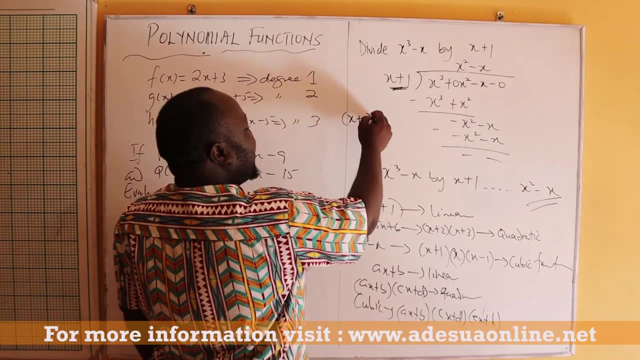 That is a cubic function. So what you see here is one factor, because it leaves a remainder of zero, okay. And the other factors, x, are x squared minus x, And you see, if I have x plus one and then x squared minus x, 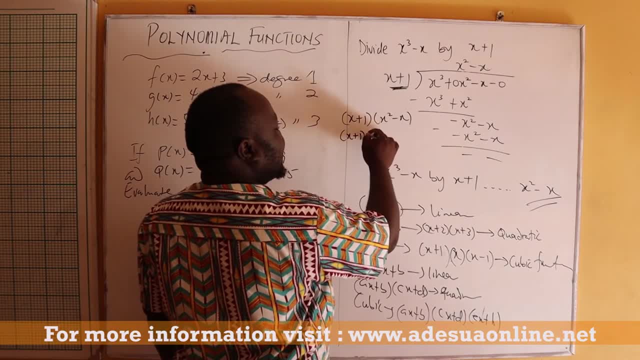 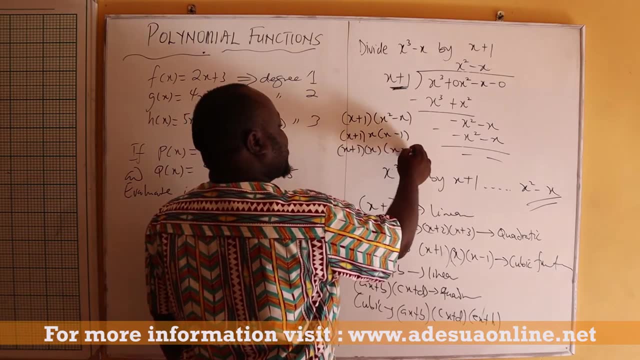 In the first one I can have x plus one. This will give me x out x minus one. okay, So I can have x plus one, x and then x minus one as my factors. So if this is equal to zero, 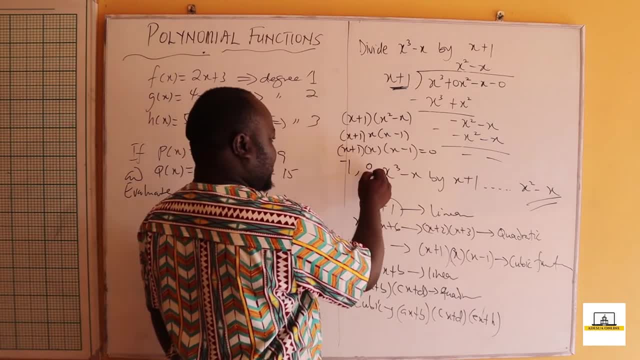 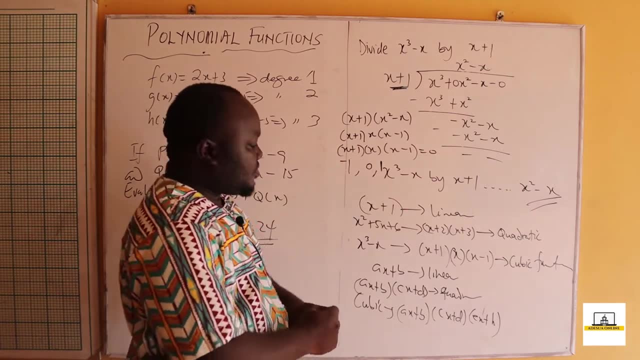 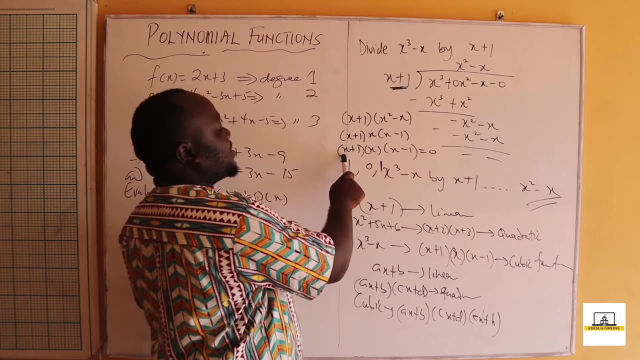 you realize that x equals to negative one, x is equal to zero and x equals to positive. one are the factors of this: x cubed minus x. So now these are the zeros of the function: x cubed minus x. okay, And the factors are x plus one, x and x minus one. 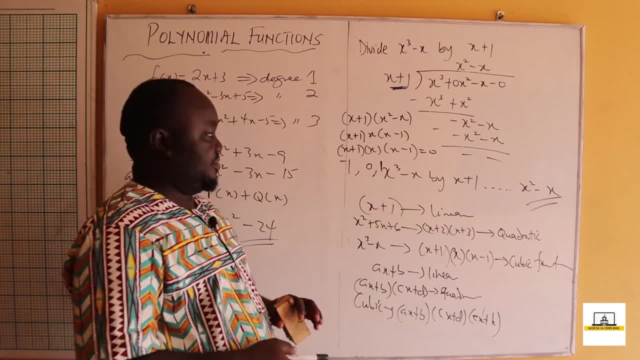 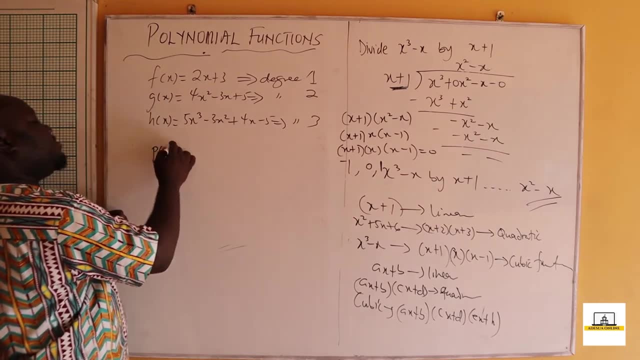 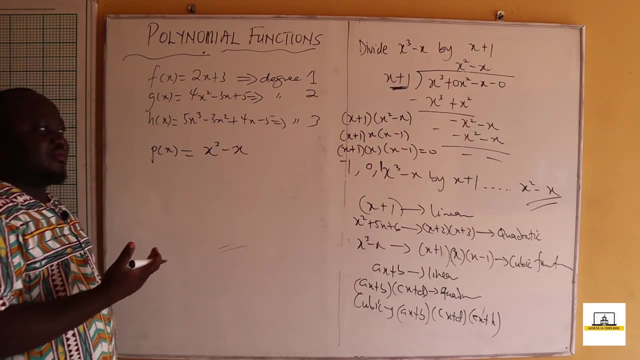 Now we have what we call the remainder theorem. Now if I have a function p of x, assuming I have a function p of x to be equal to x cubed minus x, okay, And I want to check whether, if I put one inside, 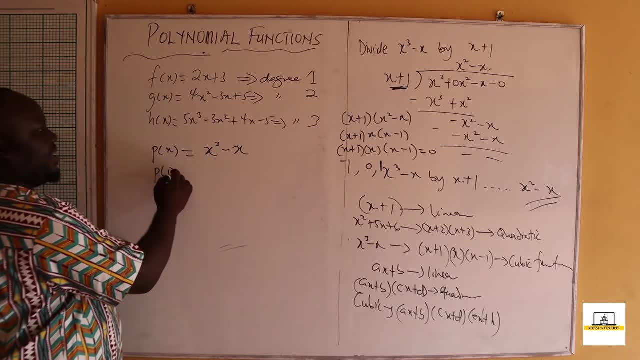 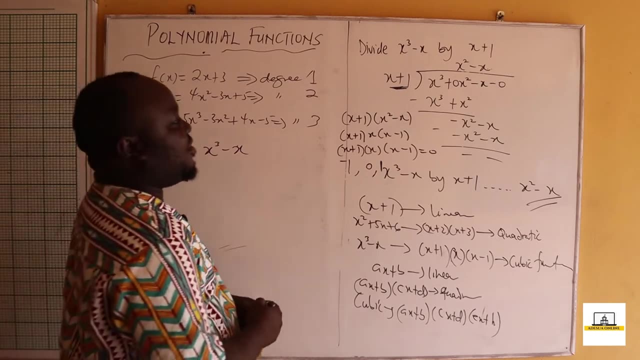 I'll get zero. you see, So if I put p of one, okay, Because even if I put p of negative one, I want to find the remainder- okay, Let's assume that I want to find the remainder of this: When I divide x, cubed minus x, by x plus one, 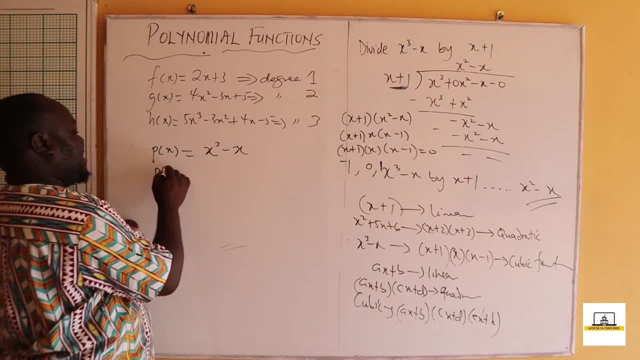 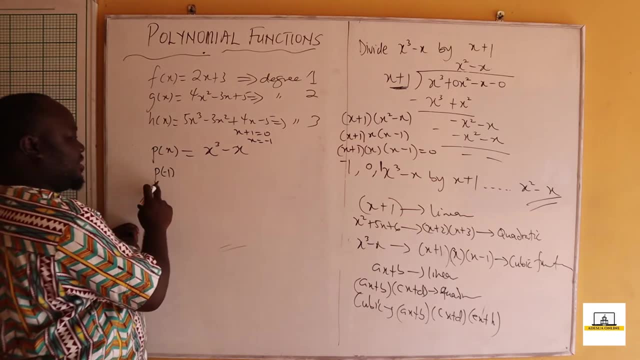 I want to find the remainder of this, So this function. so p of negative one. What is going to happen here? I put the x plus one, I equate it to zero and I solve for x to get negative one. Let's put p of negative one. 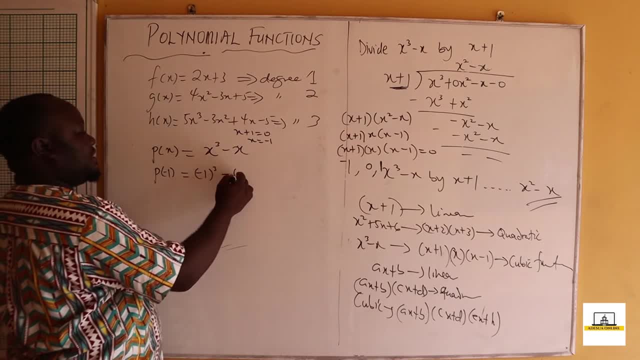 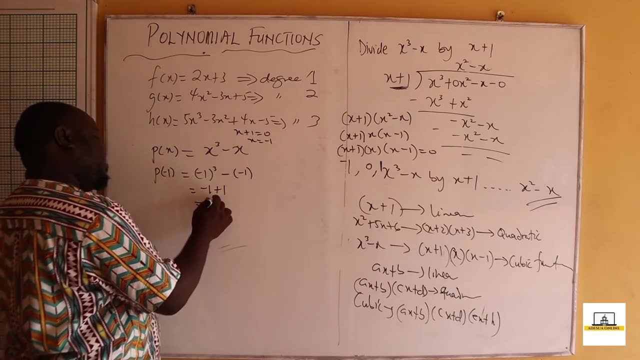 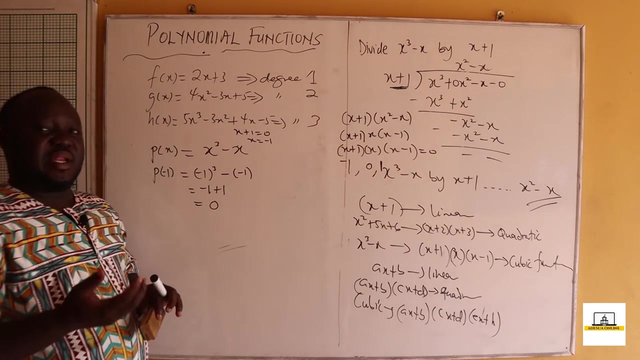 This will give me negative one cubed minus negative one. Negative one cubed is negative, one negative negative is possible plus one. This will give me a remainder of zero. We call this the factor theorem. okay, So if I want to find the remainder, 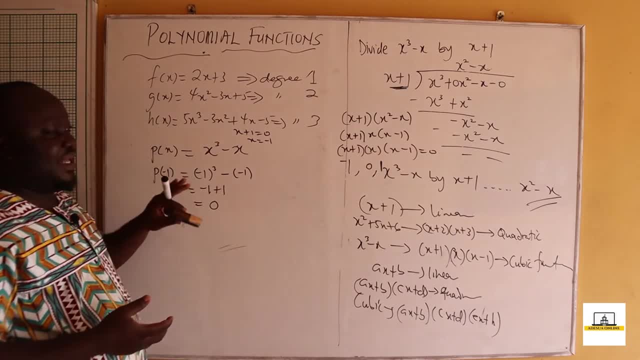 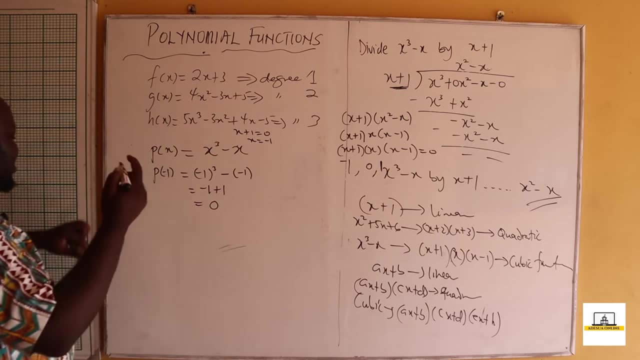 or the remainder theorem, okay, The remainder. when I divide something by something, okay, let's say a function by, let's say, a linear function. So, assuming I have p of x to be equal to 2x cubed minus 3x, 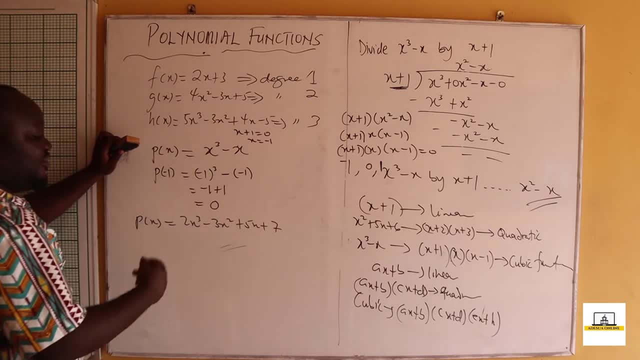 squared plus 5x plus seven, And I want to find the remainder. when I divide it with, let's say, x plus let's say two, okay, I want to find the remainder, So I just put p of what. 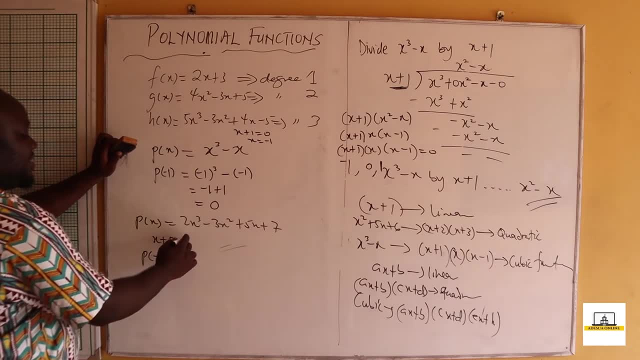 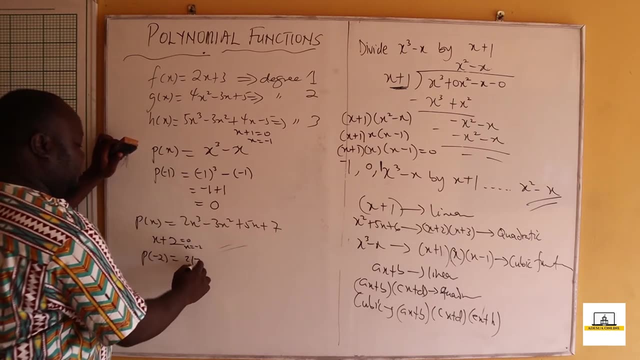 I equate this to zero, so p of negative two. So x plus two is equal to zero, x is equal to negative two. P of negative two will give me the remainder, so watch This will be two into negative two cubed. 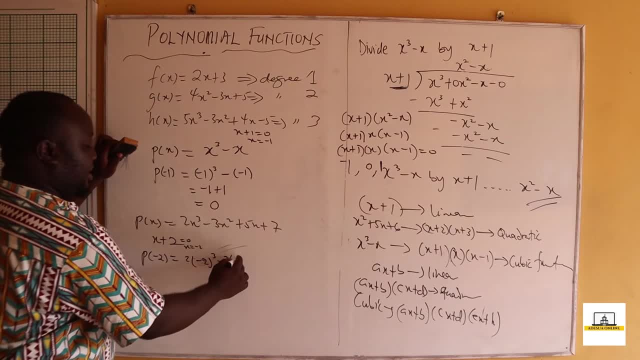 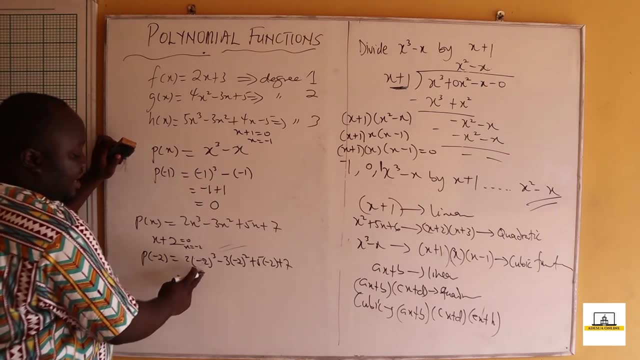 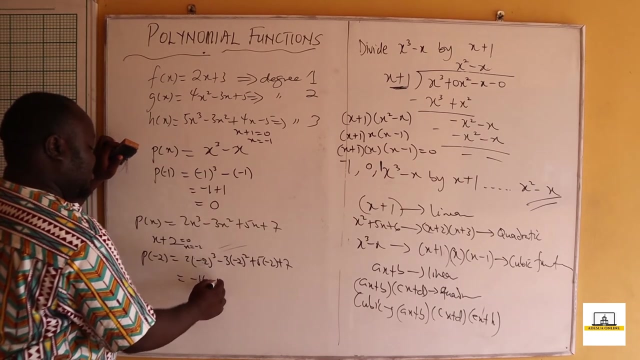 So we have two into negative, two cubed Minus three into negative, two squared plus five times negative, two plus seven, So this will give me negative eight times two is negative 16.. Then we have four times negative. three is negative 12.. 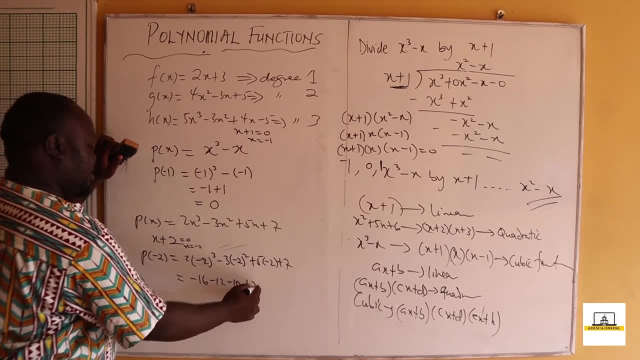 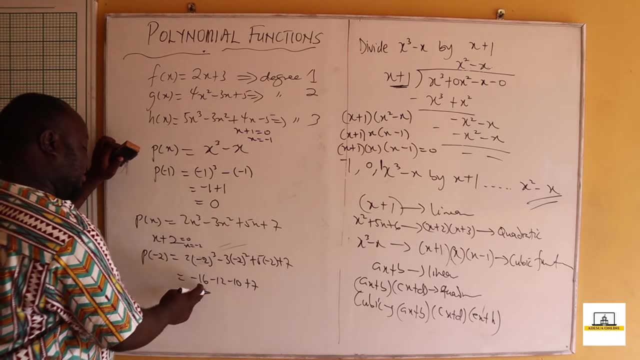 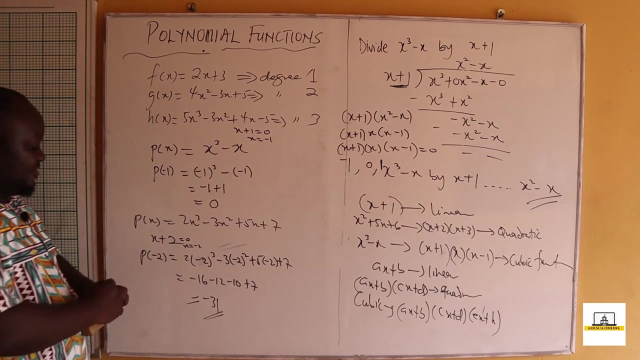 And then five times negative two is negative 10.. And I have seven. So my final answer becomes this: will be negative three negative 15, negative 15 plus negative 16 is negative 31.. So it means that if you divide two x cubed minus three, x squared plus five x plus seven, 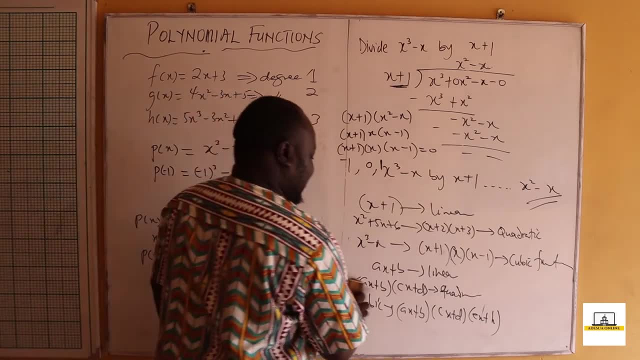 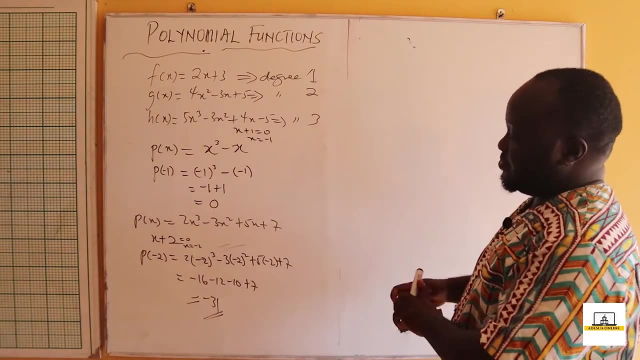 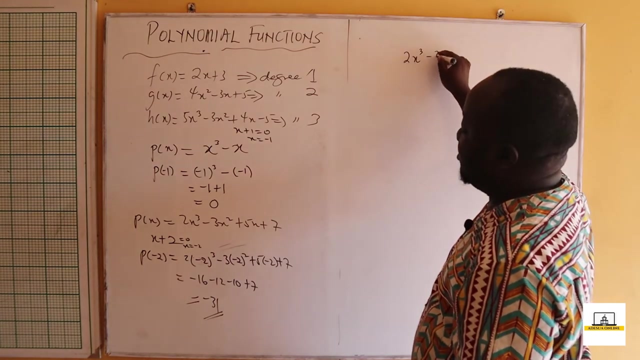 the remainder will be negative 31.. Let's find out about that. So, let's find out about that. Now I'm saying that let's divide this x plus two. Okay, we are dividing two x cubed, two x cubed minus three, x squared plus five x plus seven. 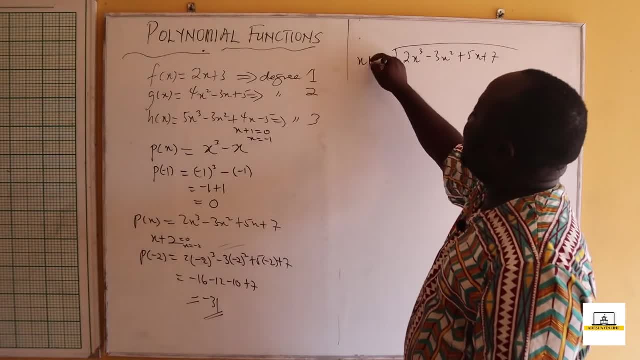 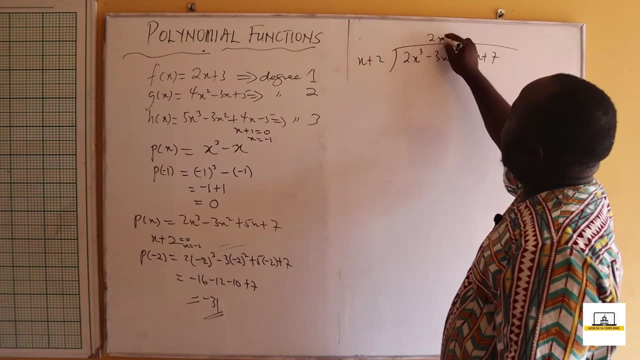 by two x. oh, x plus two. Now if this is x and this is two x cubed, what do I multiply with x to get two x cubed? You told me it's two x squared. So two x squared times x is two x cubed. 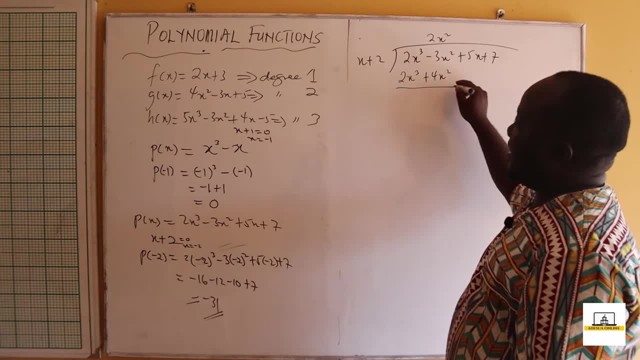 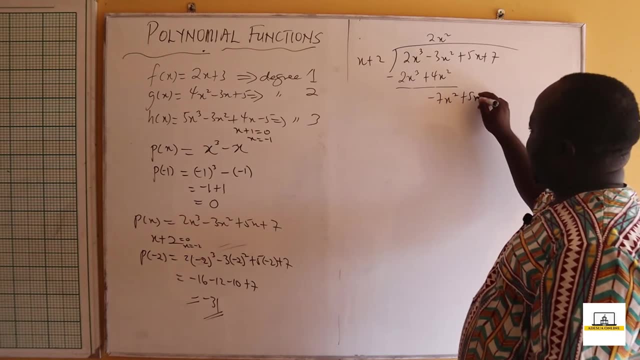 Two x squared times two is what Four x squared We subtract. this will give me zero, Minus three x squared. minus four x squared will give me minus seven x squared, plus five x. Now, if this is x and this is minus seven x squared, 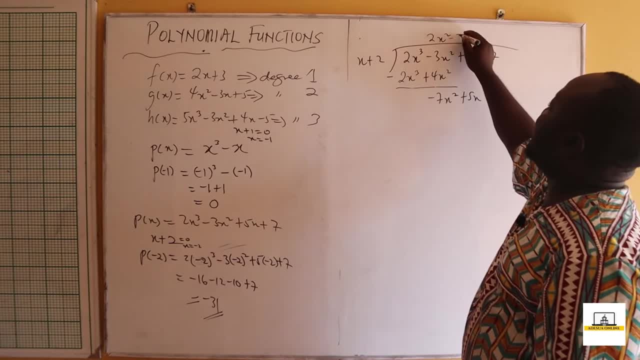 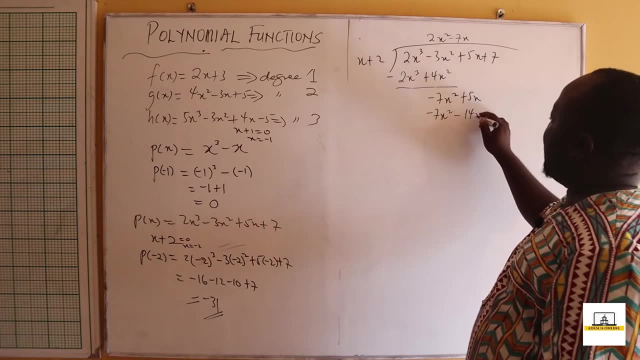 what do I multiply with x to get minus seven x squared? It's minus seven x. Minus seven x times x is minus seven x squared. Minus seven x times two is minus 14 x. Again, we subtract. this will give me zero. 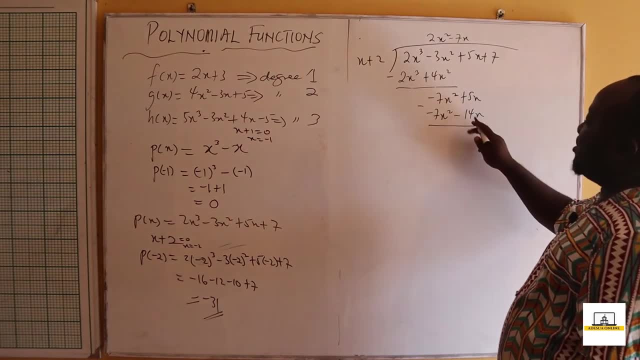 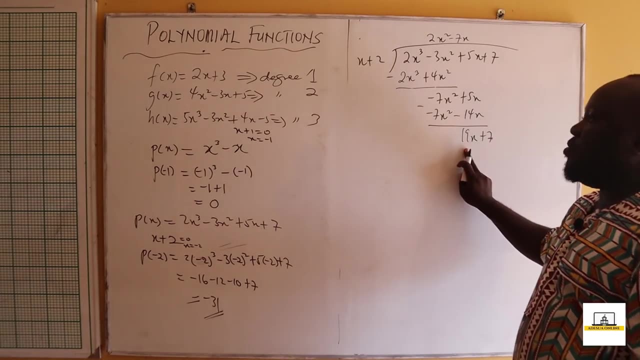 Then five minus minus 14 will become five plus 14, which is 19 x plus seven. Now, if this is x and this is 19 x, what do I multiply with 19 to get? what do I multiply with x to get 19 x? 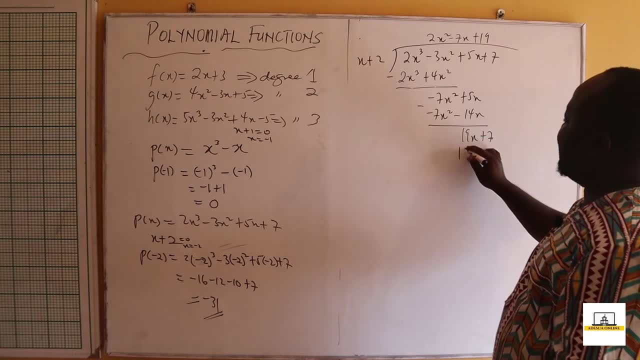 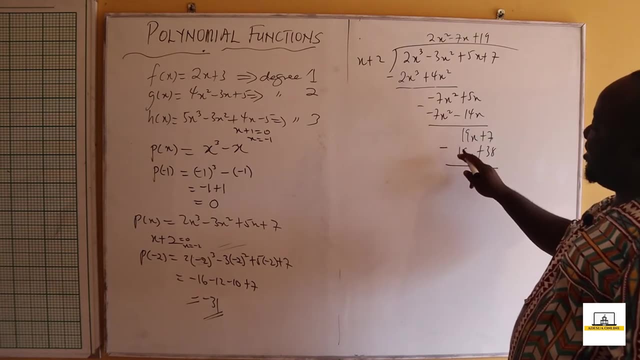 That will be positive 19.. 19 times x is 19 x 19 times two will give me 38.. We subtract Now this will be: 19 minus 19 is zero. Seven minus 38 will give me minus 31.. 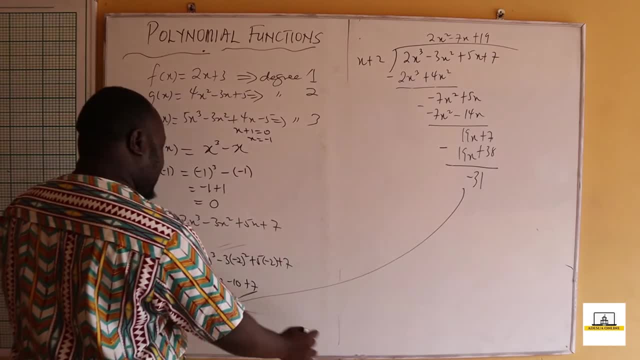 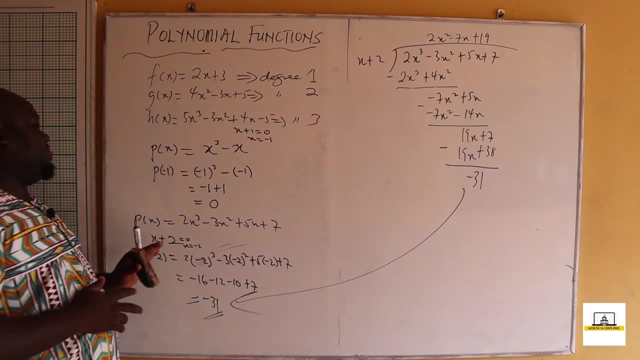 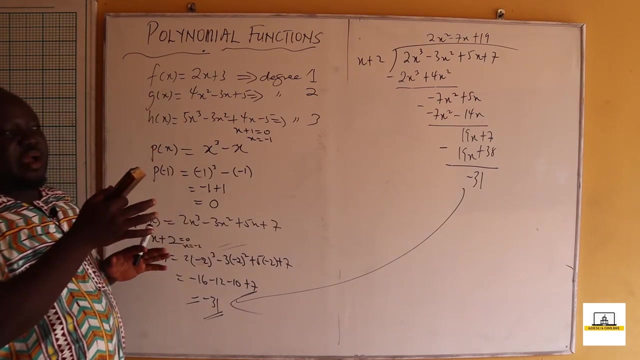 So my remainder, indeed, is equal to what Minus 31.. So you could see that for me to get a remainder is very easy. Just put in whatever you have there. If you have been asked to find a remainder, okay, you can just put the factor there. 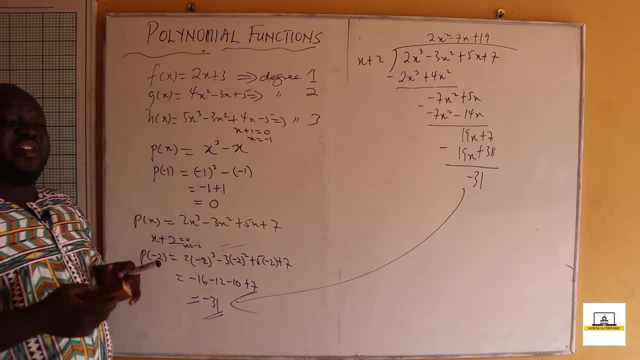 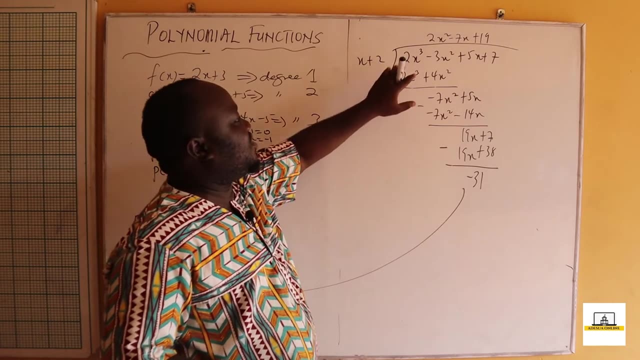 And see whether I give you a zero or not. If it gives you a zero, it means this: x plus two is a factor of this. But since we are not getting zero, it means x plus two is not a factor of this function. 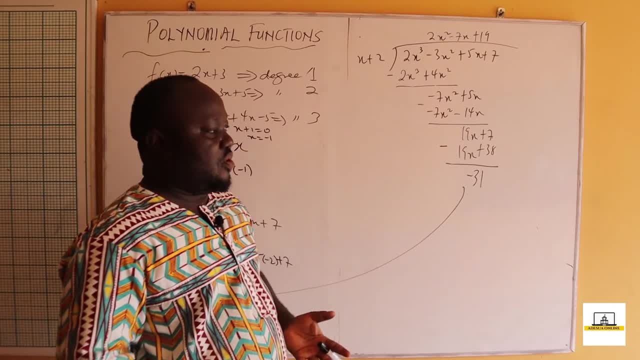 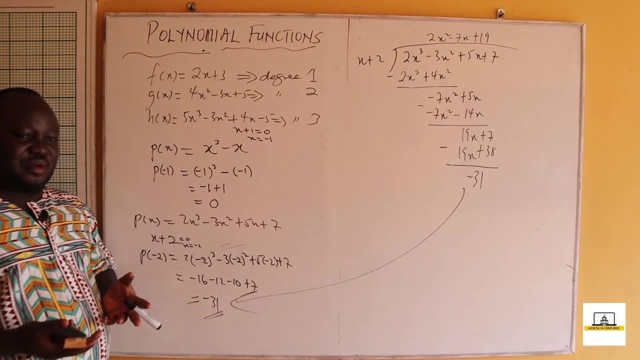 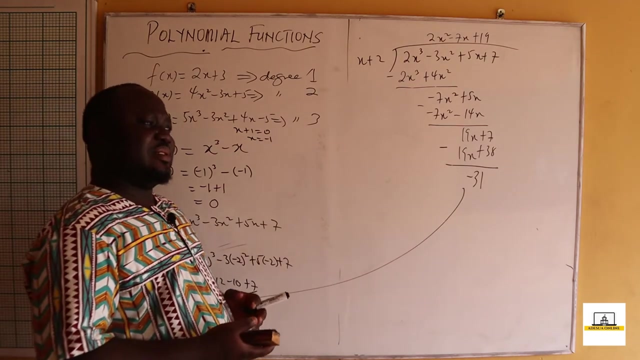 two x cubed minus three x squared, plus five x plus seven. Okay, So it leaves a remainder of what, Because it leaves a remainder of negative what- 31.. Okay, Now, when we talk about polynomials, we talk about so many things. 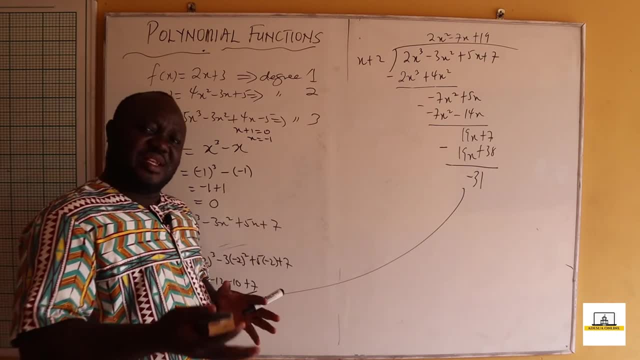 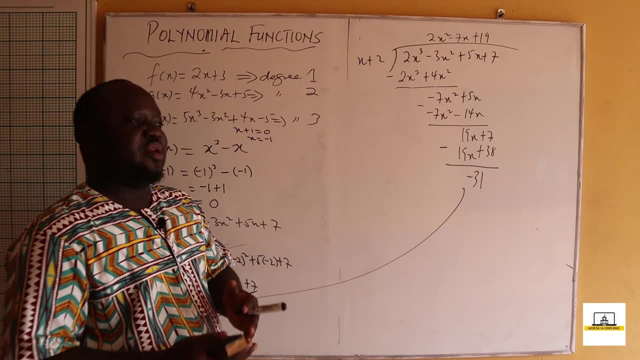 Okay, Like I said, for linear, one term: a x plus b. Quadratic, we have two terms: a? x plus b, c x plus z. For cubic, there will be three terms: a? x plus b, c x plus z. 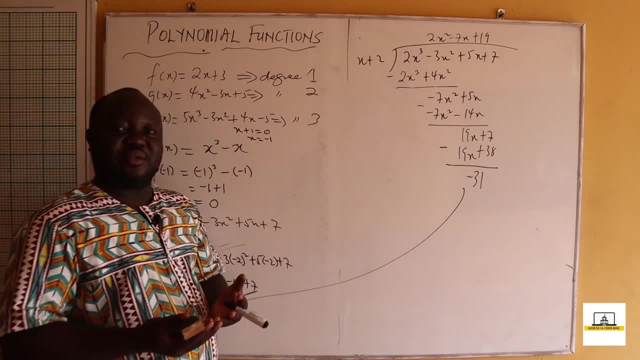 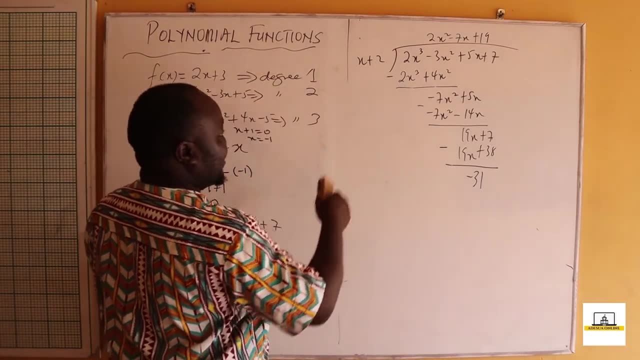 and then e x plus h. Okay, So, depending on how you are told, you can be asked to factorize a polynomial. okay, So, assuming you are asked to factorize a polynomial like this: two x cubed minus three x squared plus five x squared plus seven. 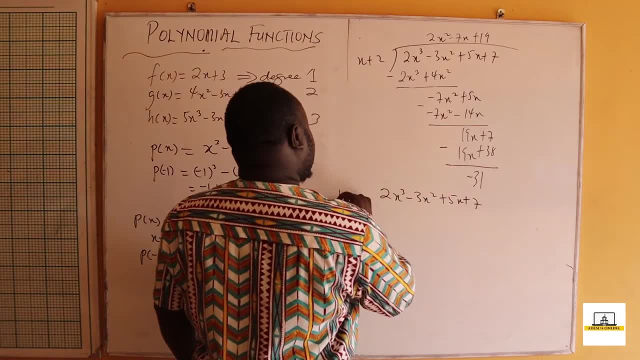 Okay, Let's say the polynomial is p of x equals to this. All you do is you are going to put in numbers here. okay, That will make you get zero. So you can start with zero negative, two, positive two, five negative five. you keep doing your try and error. 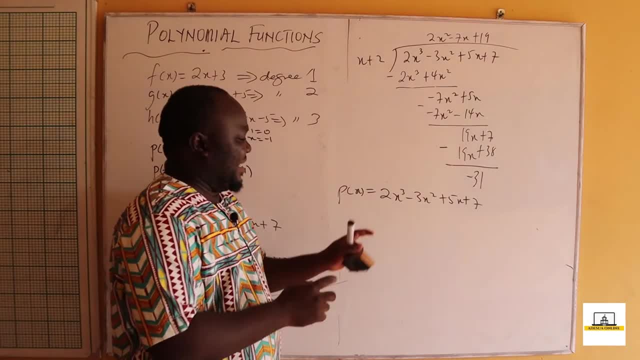 Okay. So you get a number that will give you zero. So assuming, assuming that I put p of three okay into this and I put two x cubed minus three x squared, plus five x plus seven, that would make you get zero. 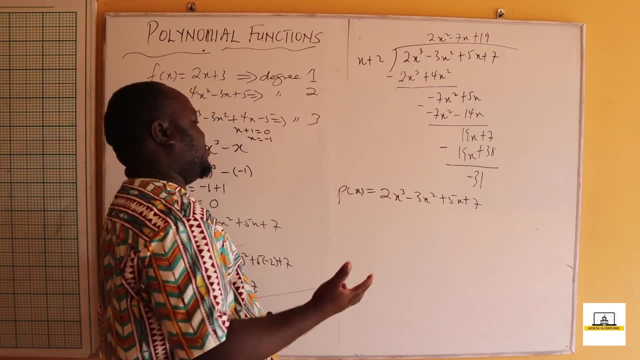 So you do this. Okay. So you have a good number and you get a number. Now for the next one, you can do this. Let's say: you have a good number and you get a number. Let's say: you have a good number and you get a number. 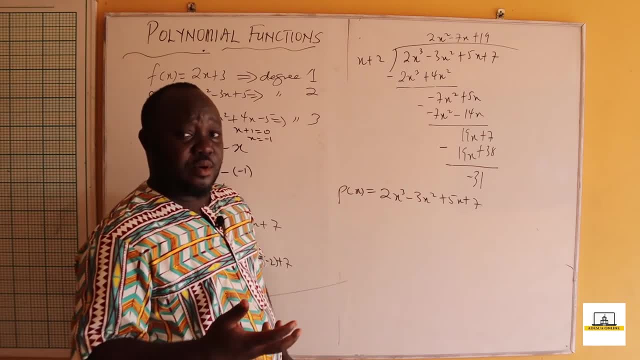 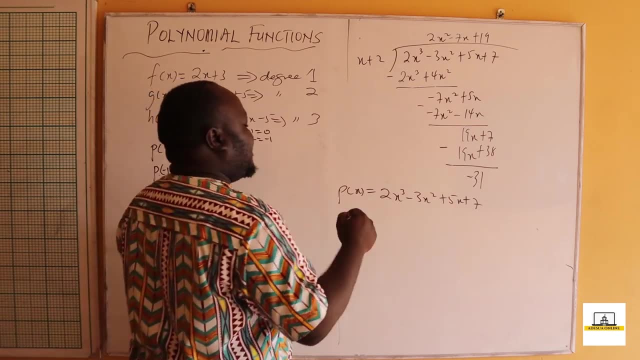 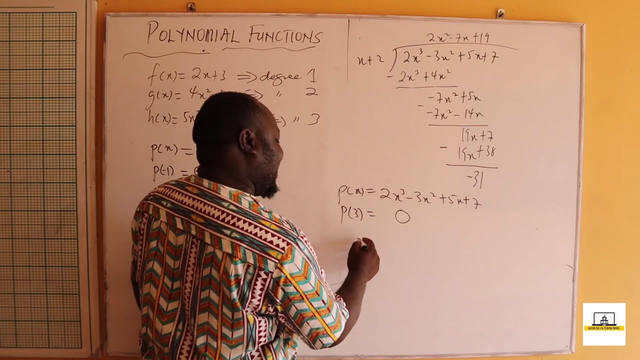 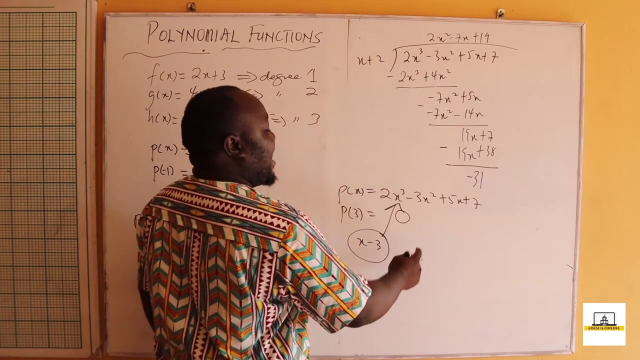 Okay, So you have a good number and you get a number. I realize that I get 0,. okay, It means that x minus 3 is a factor of this polynomial. okay, And since x minus 3 is a factor, I'll just divide this with x minus 3. 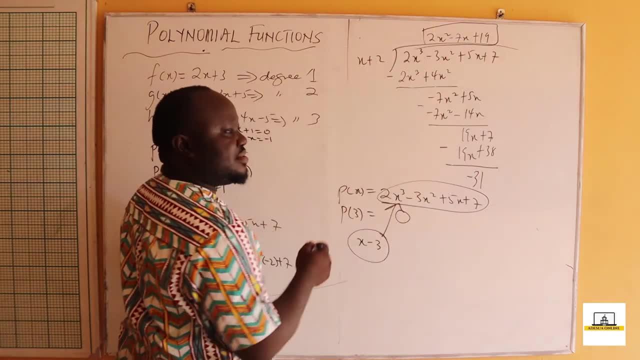 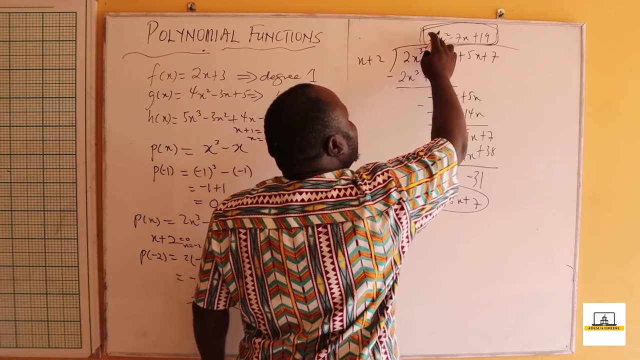 to get the other factors over here, which would be my quotient, okay, And when x minus 3 is a factor and getting my quotient, I also factorize my quotient, which is in the form of what A quadratic expression? okay? 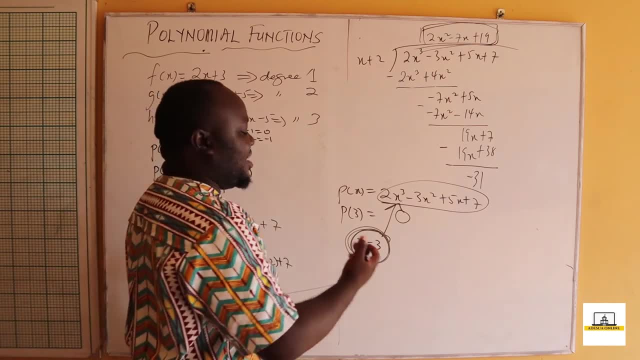 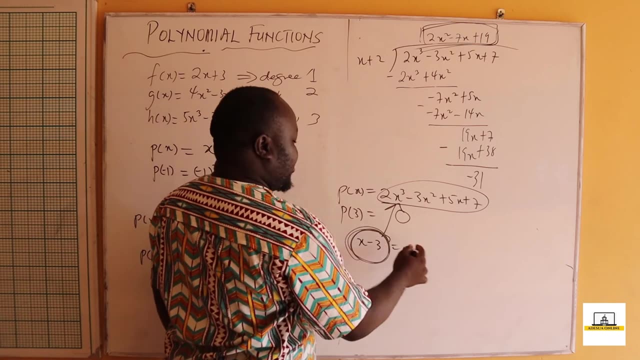 I also find, factorize it and then that will give me the other factors. If you are asked to find the zeros, it means you are going to equate this to 0, and this also to 0, and then factorize it and then equate it to 0. 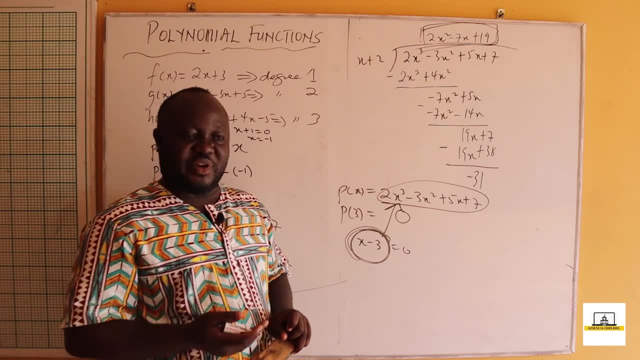 and get your zeros of what Your polynomial, or zeros of your function. So let's pick an example and solve. 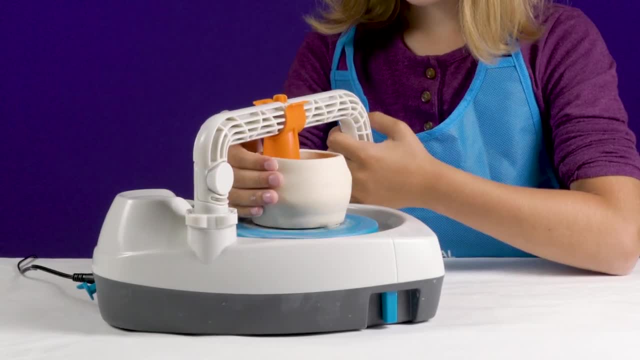 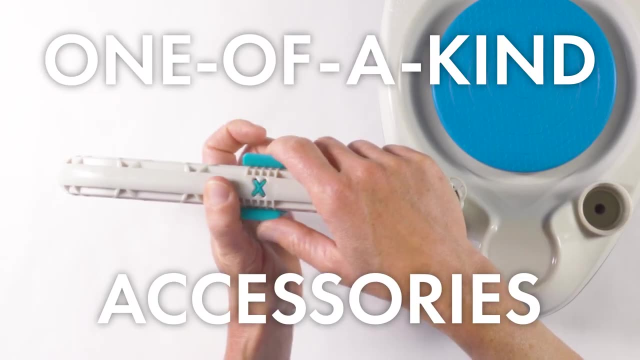 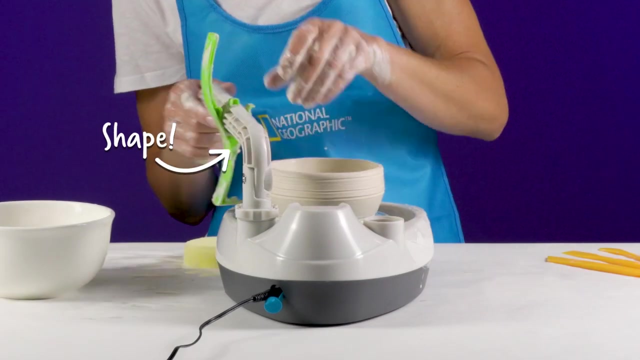 Make amazing bowls, cups and more with a National Geographic Explore Series Pottery Wheel. Learn to form clay with one-of-a-kind accessories, like our revolutionary tool arm and shaping attachments. This pottery wheel has everything you'll need to shape and decorate your pieces.